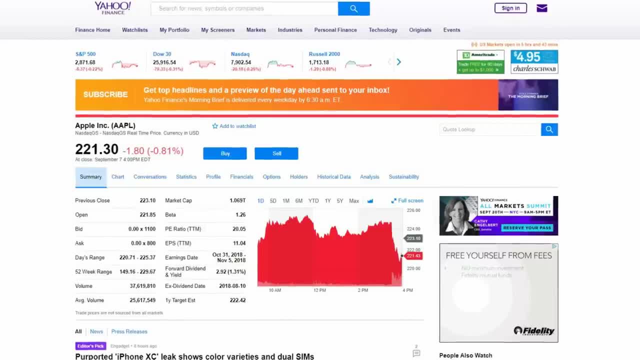 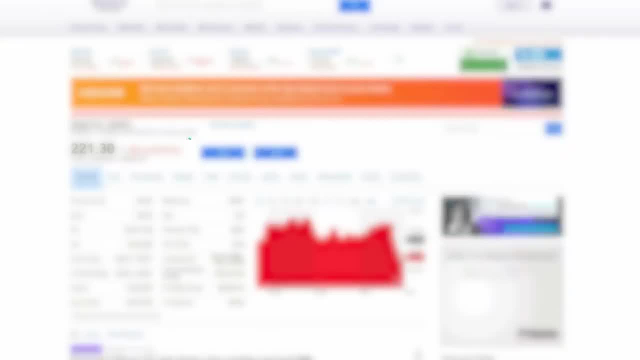 It means the last time someone bought or sold this stock, they did it at the price of $221.30.. Both the buyer and seller agreed to transact at that price. This is usually the price people are talking about when they see the stock price went up or down. 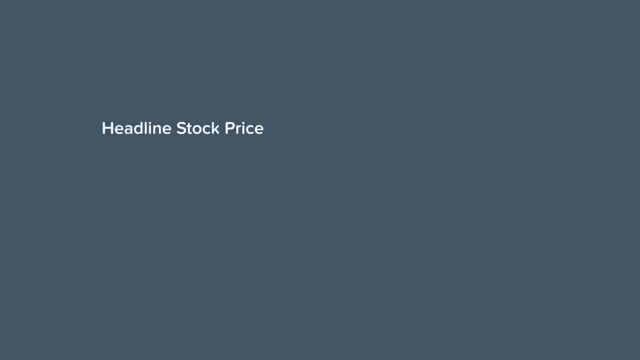 To be absolutely clear, the headline price quoted on the market is not the stock price at which you can buy the stock at that particular moment. That's a common misconception. It's the price at which you can buy the stock at that particular moment. 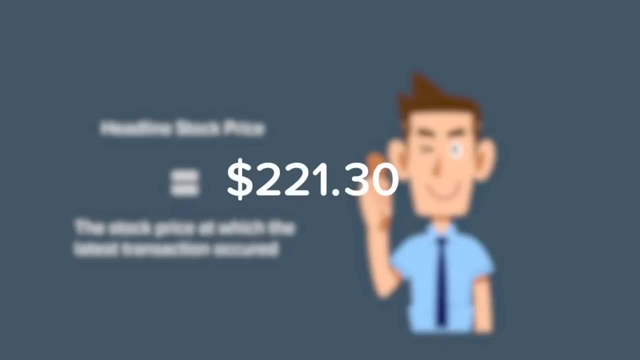 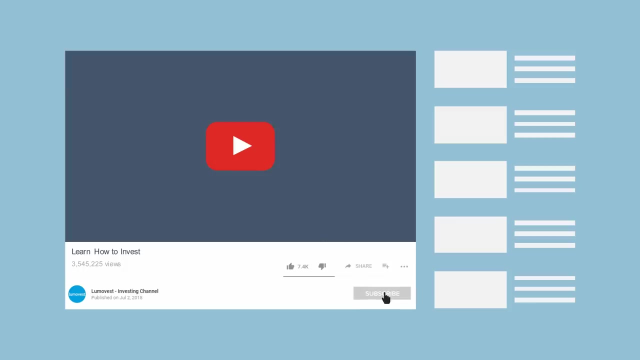 If we were to buy it, it could be $221.30,, but it'll probably be somewhere pretty close to it, Maybe $221.29 or $221.31.. It wouldn't necessarily be exactly at that price. By the way, we make new videos on investing in personal finance every week. 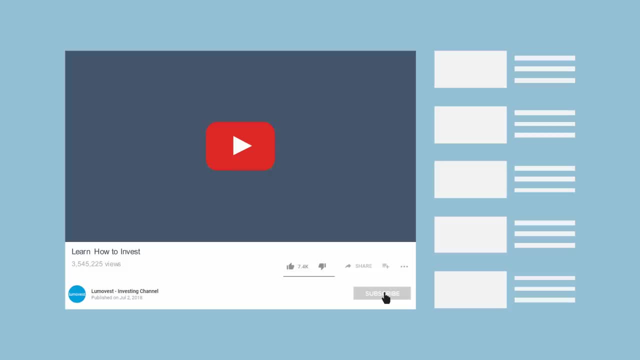 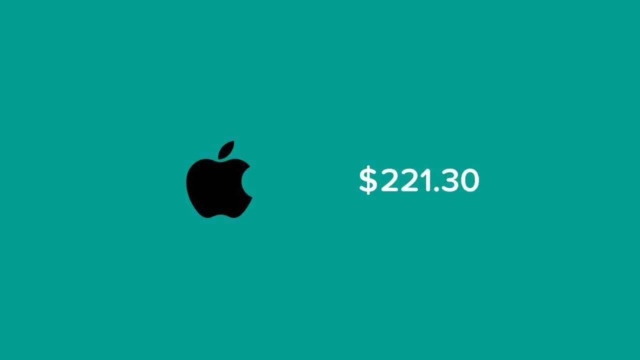 so if you're new to Lumovest, consider subscribing to our channel. Naturally, this raises the question: how do people know to buy or sell the Apple stock at $221.30? Why not $100 per share or $400 per share? 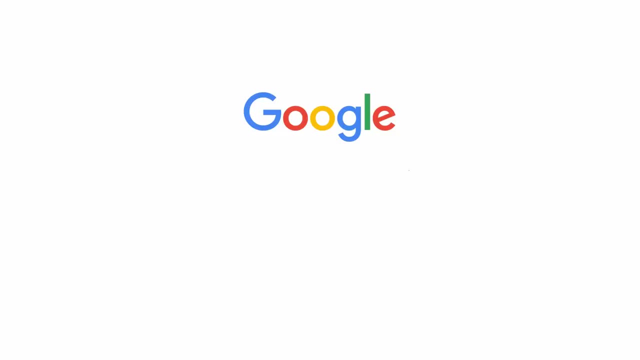 How did they zoom in around the $220 range? If you do a search on Google or YouTube, you'll hear people say that the stock price is driven by supply and demand. That's true, but that's also very vague, Like what's guiding the supply. 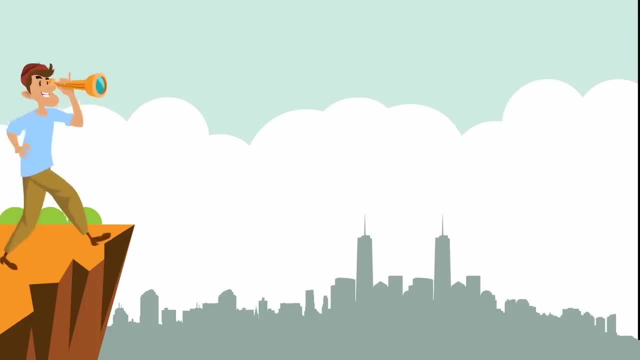 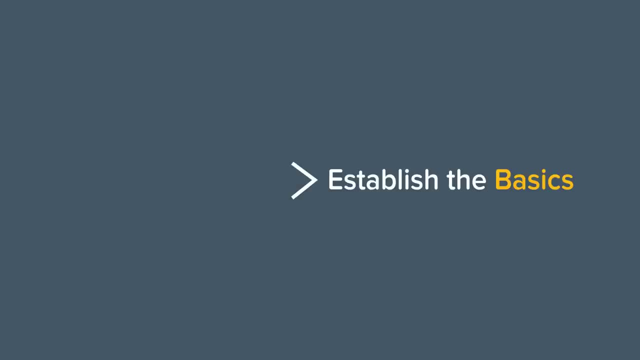 and demand for a particular stock. So we're going to demystify everything here and show you how to buy a stock at $221.30.. Let's start with the basics. Let's start with the basics. Recall that when you buy stocks, you're buying pieces of ownership in the business underlying. 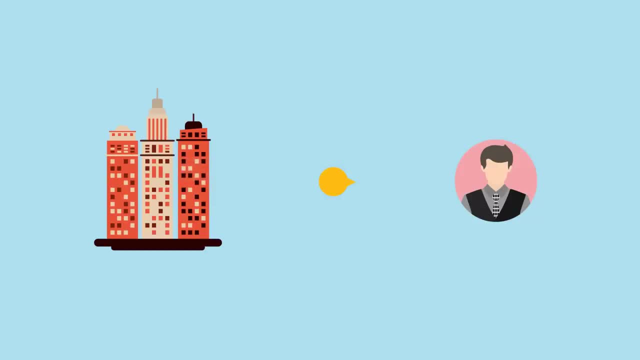 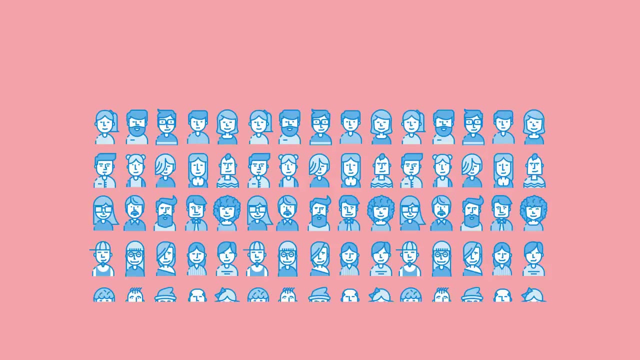 the stocks, You'll become one of the owners or shareholders of the company. If you didn't know about this, check out our other video explaining what a stock is. Publicly traded companies could have millions of shareholders each owning a small piece in the company. Take Apple, for example. 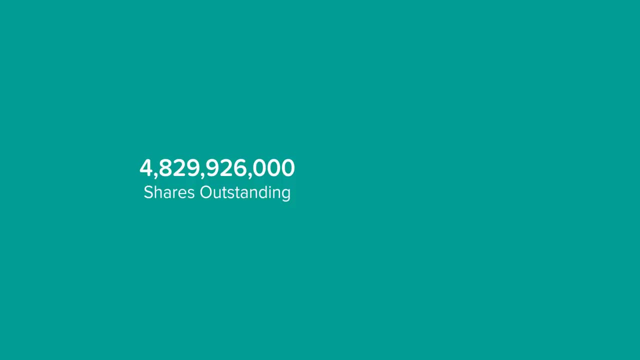 Apple has 4,829,926,000 shares outstanding. If you purchase 10 shares, you'll own 0.0000002% of the company. You might own a very small piece of the company, but you're a business owner nonetheless. 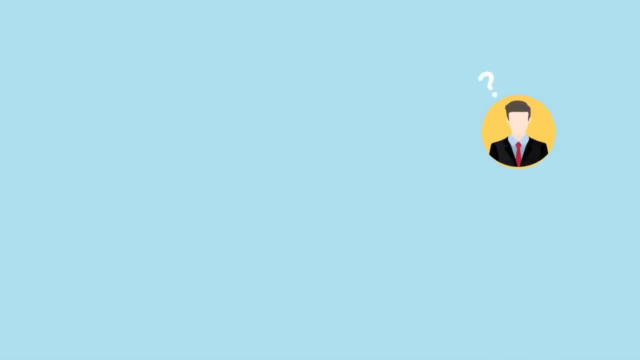 So let's think about owning a business. How do business owners make money? They make money when the companies they own succeed in commerce and earn lots of cash from selling their products and services. The cash we're referring to here are the cash that can be given back to the business owners. 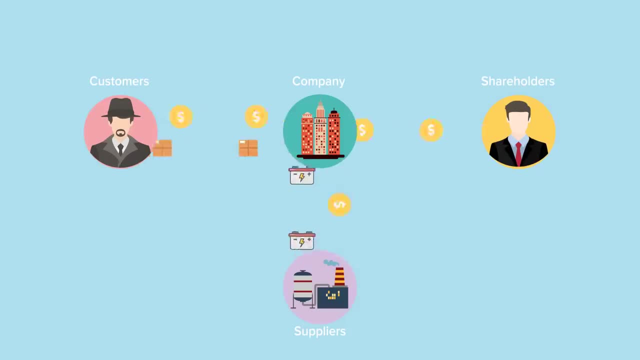 after paying for all the expenses and reinvestment needs. This is known as free cash flow Cash that the business is free to give to their owners because all the necessary expenses have already been paid for. Business owners can then use that cash to buy whatever they want. 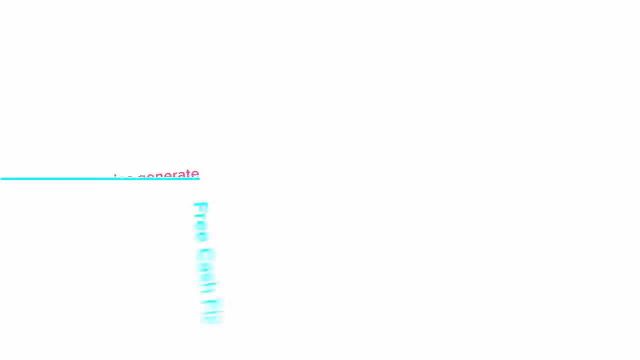 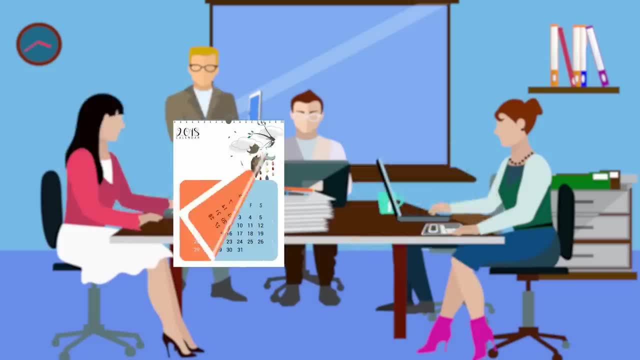 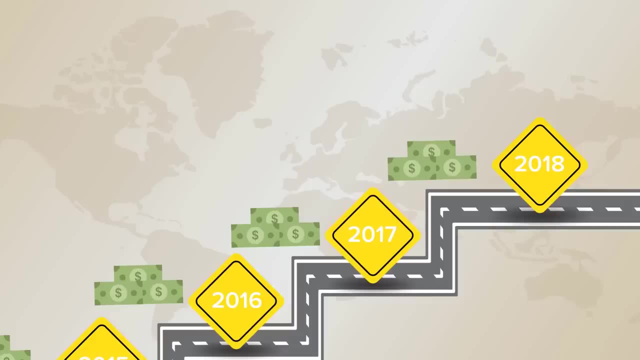 This year, the next year, the year after that, all the way into the future. So essentially, as a business owner, you're entitled to the free cash flow that your company will earn through the remainder of its lifetime If you owned 100% of the business. guess what? 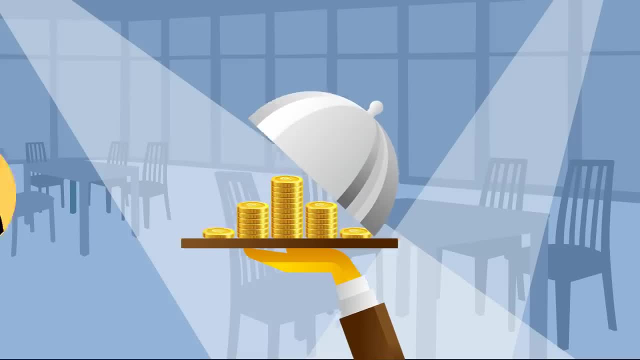 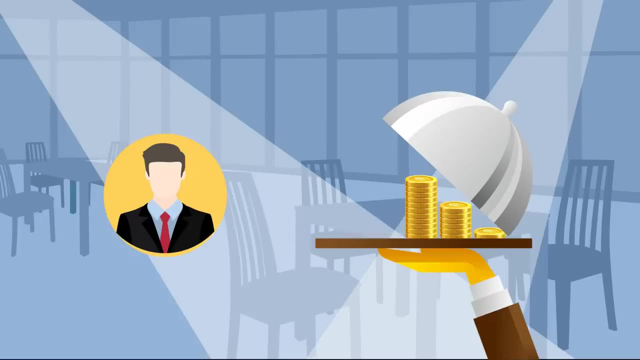 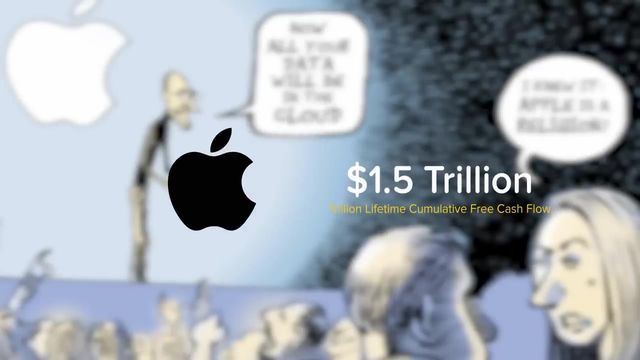 all that future free cash flow would belong to you, But because you don't own 100% of the business, you're really only entitled to a piece of that free cash flow Equivalent to your ownership interest. Say you believe Apple will generate 1.5 trillion dollars in cumulative free cash flow. 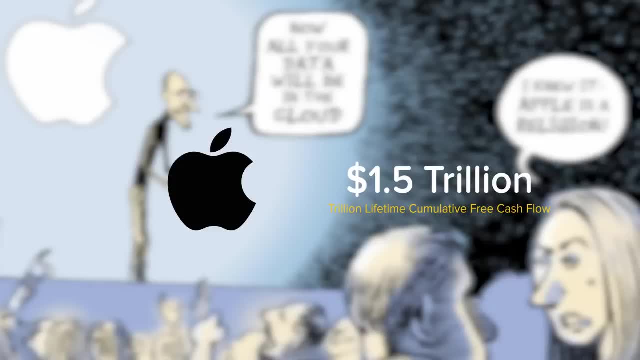 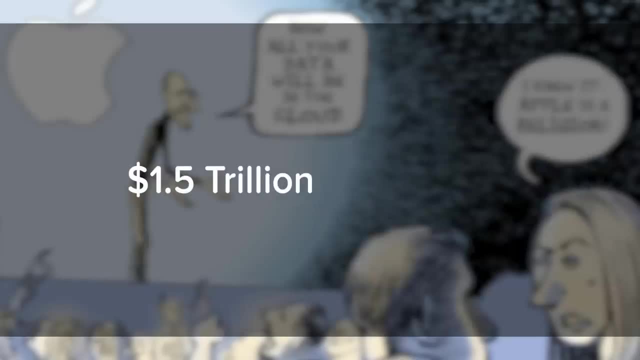 over its lifetime, that it will give back to you all at once. We just arbitrarily made that number up to illustrate as an example, But let's assume for now this is the case. That's 1.5 trillion dollars that can be given back to us shareholders in the future. 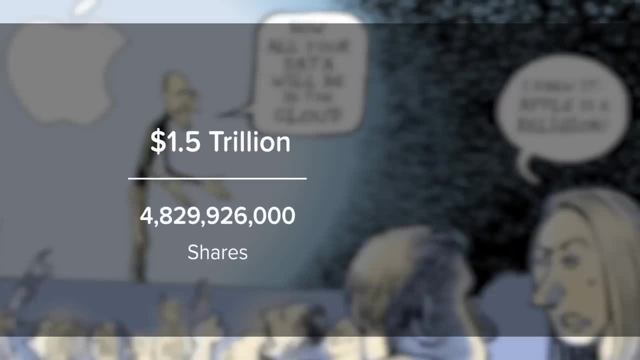 Well, divide that by 4 billion 829 million 926 thousand shares and you get $310 for every share that you own, Meaning that each share is entitled to getting $310 back over Apple's lifetime. This $310 is known as future value. It's the money you'll get from the future free cash flow. 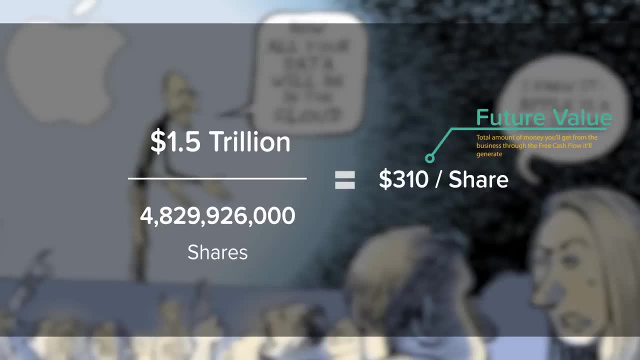 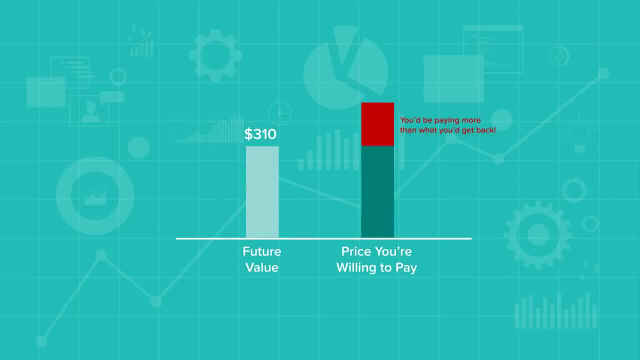 that the business will generate over the remainder of its lifetime. Naturally, in this example, you would never want to pay more than $310 for an Apple stock, because otherwise you'd be paying more money than what you get back in return. That's like saying: 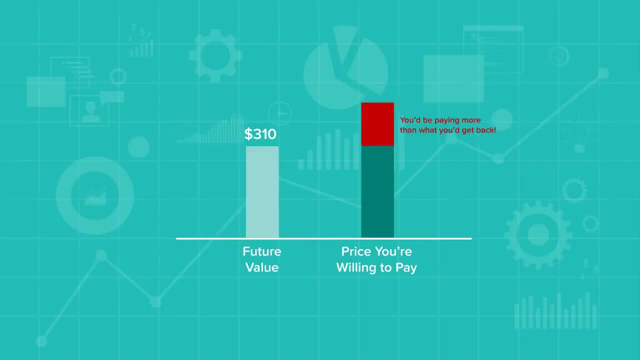 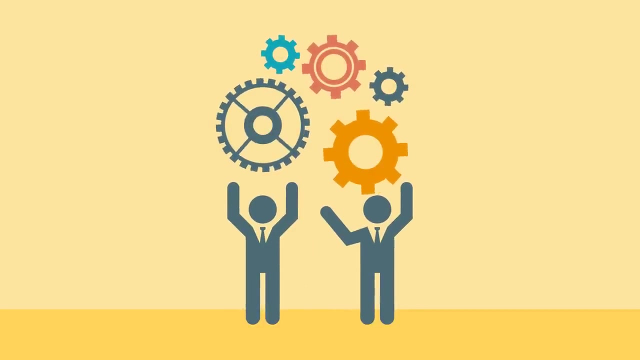 you want to pay $20 to buy a $10 bill. so at this point in your analysis, you know that you wouldn't want to pay more than three hundred and ten dollars for the Apple stock. a price below three hundred and ten dollars could potentially make sense, but the logic doesn't stop here. there's more to it. that's because you're 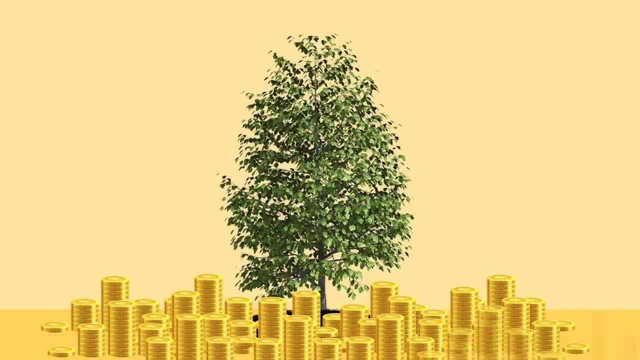 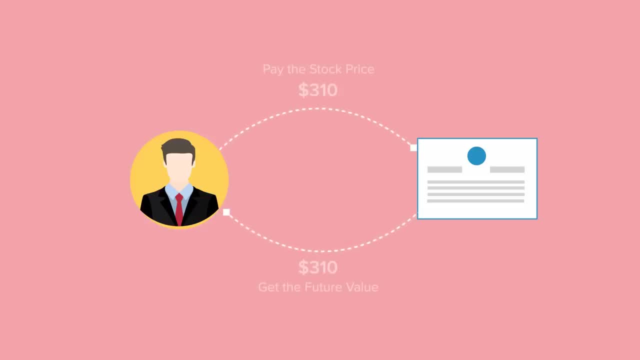 not getting the future value right after you invest in the Apple stock, you get it in the future. as an investor, you're looking to make a profit. you're not looking to buy a stock for three hundred and ten dollars today. that will give you the same three hundred and ten dollars in the future- your wealth. 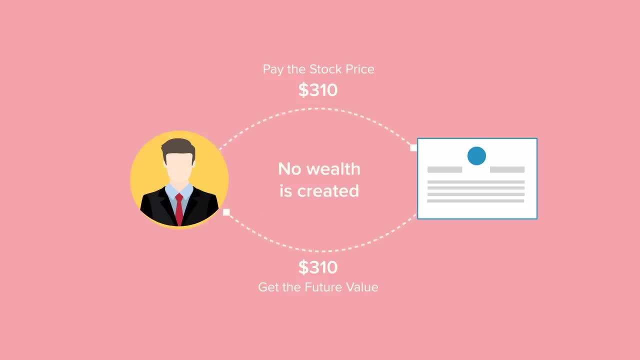 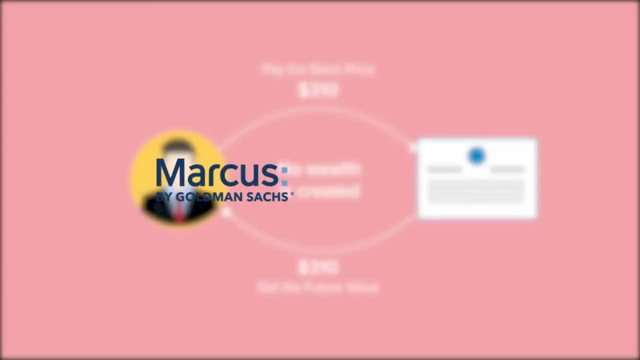 wouldn't have changed and that'd be a pretty meaningless investment. you'd be better off to just hold on to the three hundred and ten dollars and put in the bank. with Goldman's online savings account at least, that three hundred and ten dollars will increase by about two percent a year. no, you want to make a. 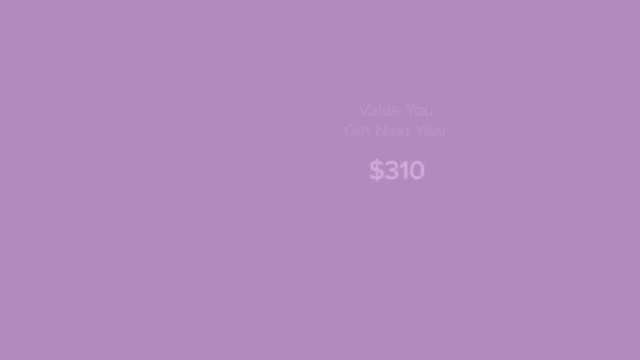 return on your investment for taking the risk of owning a business. so you have to work backwards. let's again, first, simplicity's sake, assume that Apple will give you the three hundred and ten dollars next year, so all the cash that it will ever make in the future. it'll. 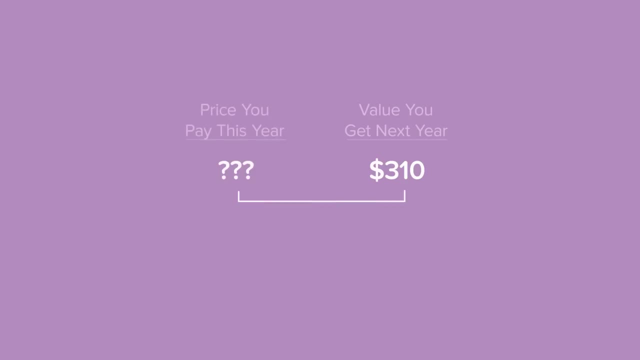 just give it to you next year- probably not going to happen, but let's assume that's the case and you determine that you would require a ten percent return to invest in this stock and to bear the risk of holding on to it for the year, then the maximum price you'd be willing to pay for it should be three hundred and 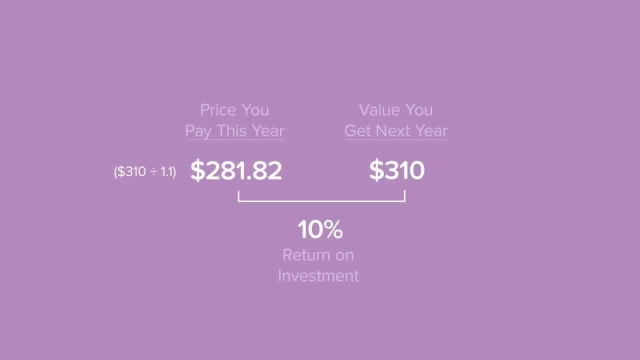 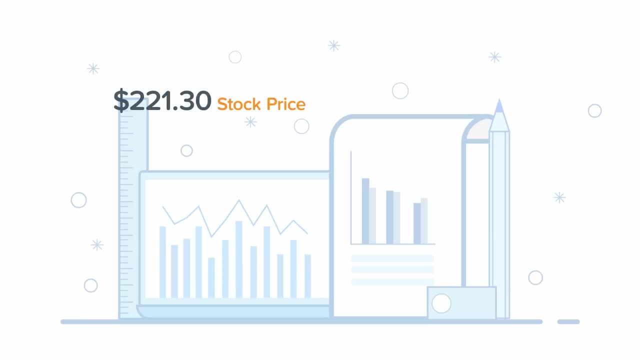 ten divided by one plus ten percent, or about two hundred eighty one dollars and eighty two cents. that way, if Apple give you back three hundred and ten dollars in cash next year, you've earned a ten percent return on your investment- pretty good. whereas the two hundred twenty one dollars and thirty cents is the stock price and the. 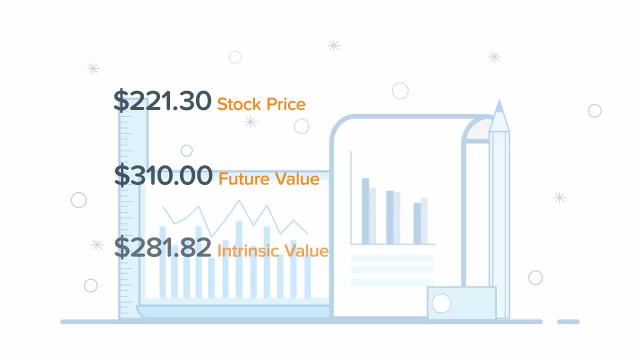 three hundred and ten dollars is known as the future value. this two hundred eighty one dollars and eighty two cents is what's known as the intrinsic value. when you hear people say you have to buy stocks at prices below the true value, they're referring to this intrinsic value. investors do their own. 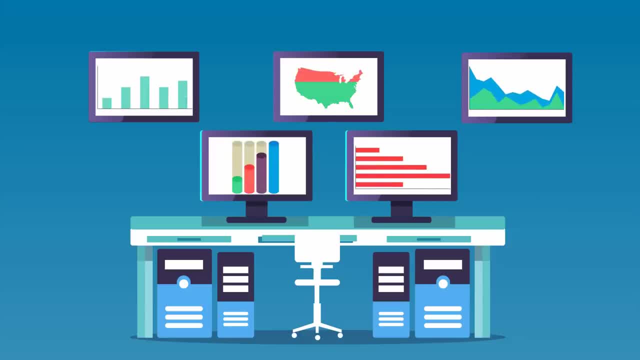 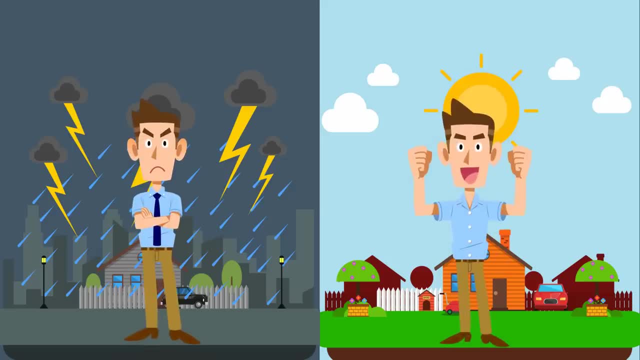 analysis and form an estimate on what they believe is the intrinsic value of the stock, and they'll come to different conclusions. some might be more optimistic about a company's future and some might be more pessimistic. investors estimate of the intrinsic value essentially guides the price that they 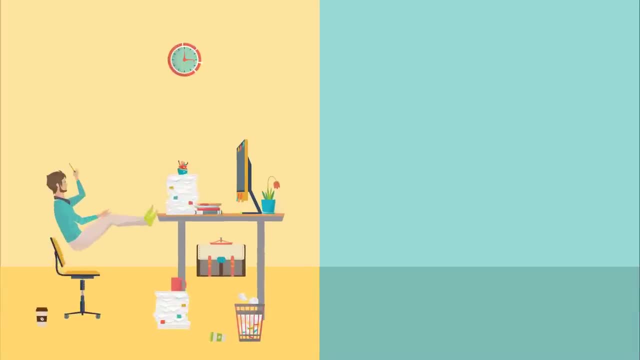 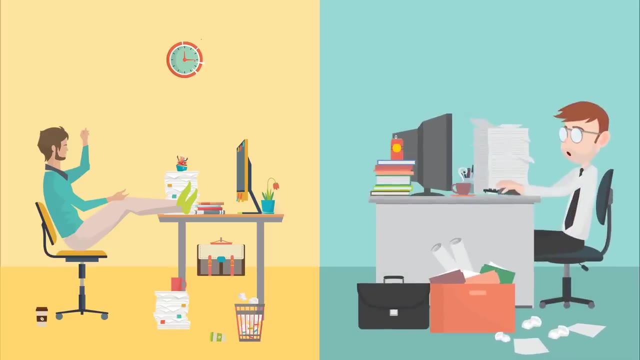 would be willing to pay. some investors, especially the retail investors, would skip over this analysis, which is a huge mistake. but the institutional investors deploying hundreds of millions to billions of dollars are definitely going to calculate the intrinsic value before they buy any stocks. these institutional investments are usually large in size and their 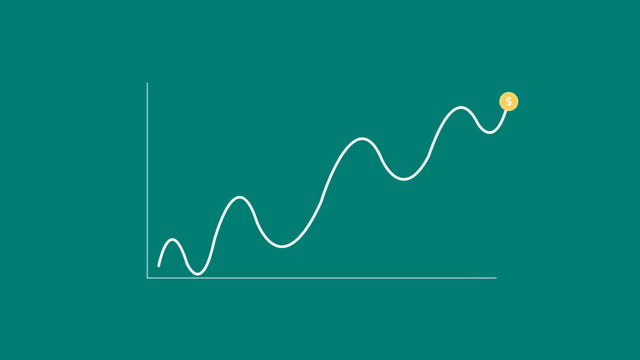 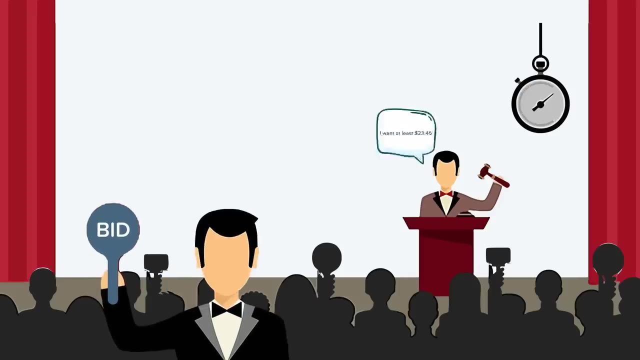 demand to buy or sell a stock will affect the stock price. once investors have a sense of the stocks intrinsic value, they then bid to purchase the stocks at prices they're comfortable with. similarly, current shareholders who are looking to sell their shares will ask for prices that they think are fair. 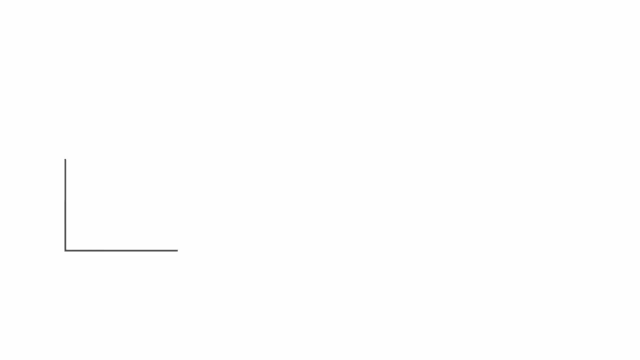 given the estimated intrinsic value. if investors believe the current stock price is way below the intrinsic value, then there would be more demand to buy the stocks and this buying pressure will bid up the stock price. likewise, if investors believe the current stock price is way above the intrinsic value, 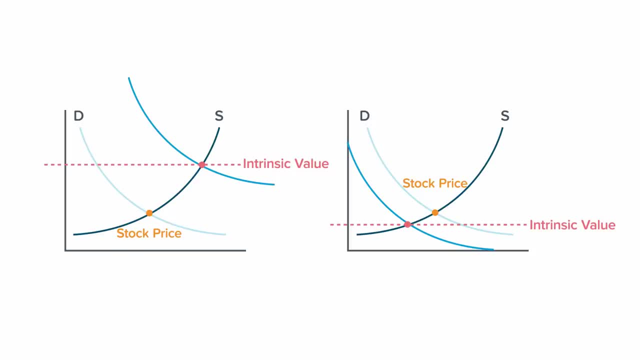 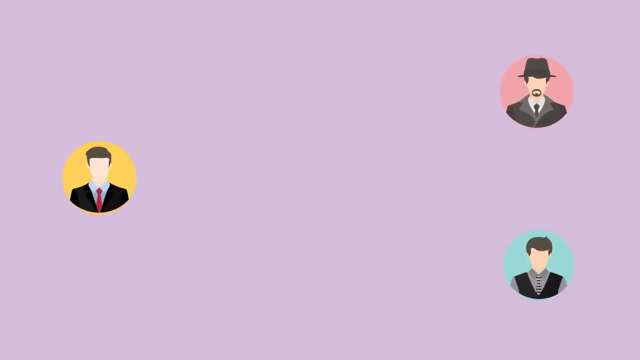 then they would want to sell before other people in the market realizes and the stock price falls. this selling pressure pushes down the stock price. so, for example, someone might estimate Apple's intrinsic value to be about two hundred and forty dollars and bid for two hundred and twenty two dollars and 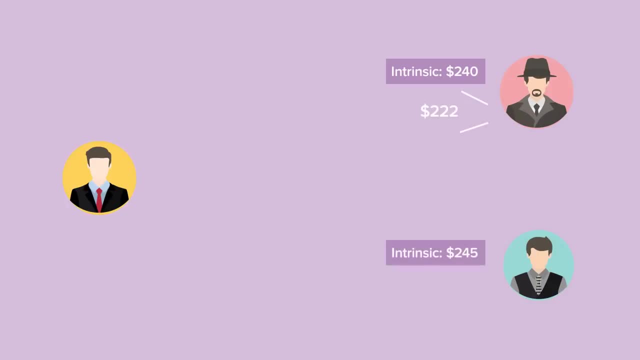 the sellers might be doing their analysis and figured it to be closer to two hundred and twenty dollars, and decided to sell their shares to the buyers at two hundred and twenty three dollars, once they transact the stock price quoted in the market changes to reflect this latest price, at which the 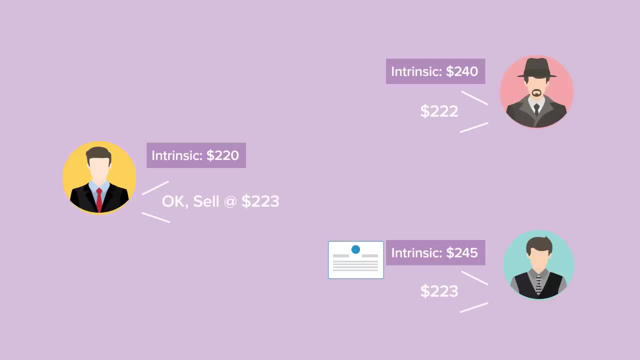 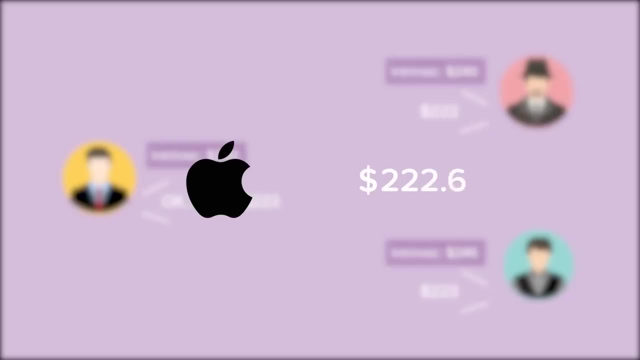 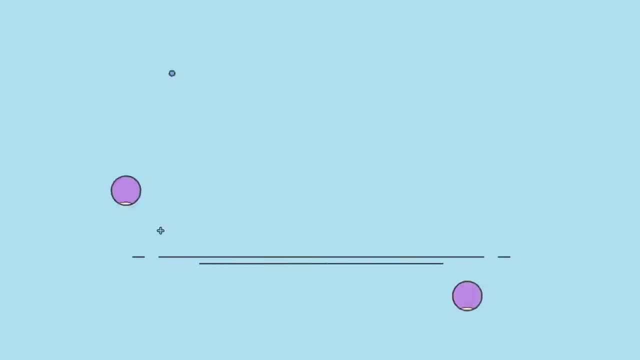 stock exchanged hands. in this case, the stock price would jump from two hundred twenty one dollars and thirty cents to two hundred twenty-three dollars and twenty three dollars and fifty cents if investors made a major assets trading to $223.. At any given moment, there are thousands and thousands of buy and sell orders with different 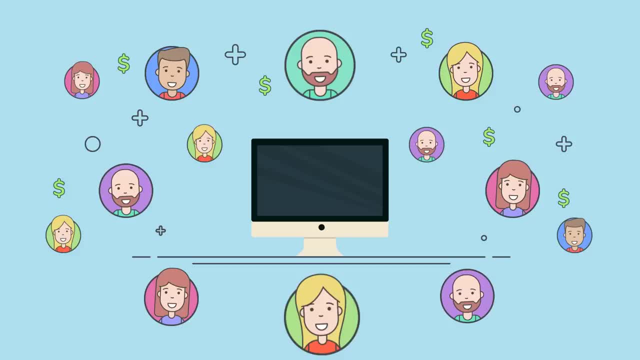 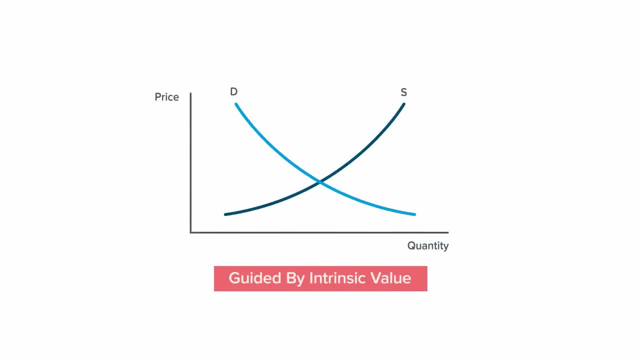 quantities of shares and prices. so it's all processed electronically by computers that match buyers with sellers. That's the market supply and demand dynamics at play, guided by intrinsic value Over the long term as more and more information come out about how much money companies are. 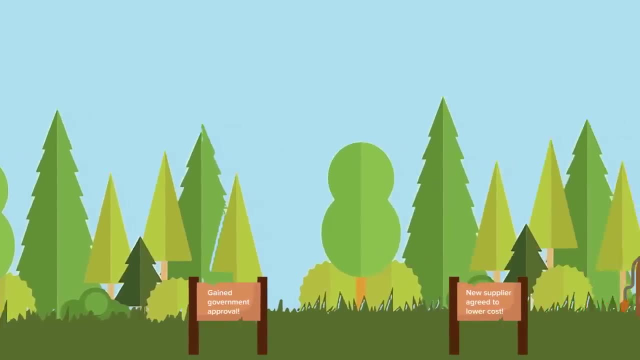 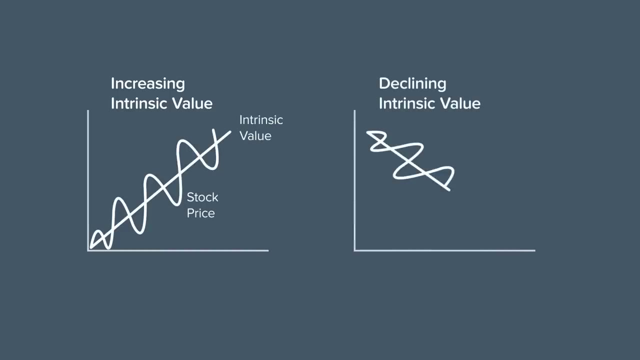 making. the stock price follows the intrinsic value. Businesses with increasing intrinsic value over time will similarly see an increasing stock price. Businesses with a declining intrinsic value will see their stock price drop. Intrinsic value is the guiding force for stock price over the long term. 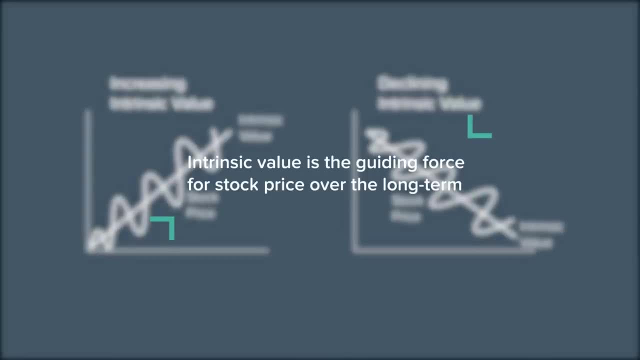 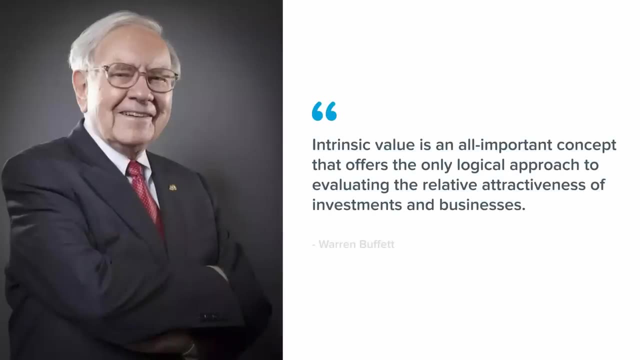 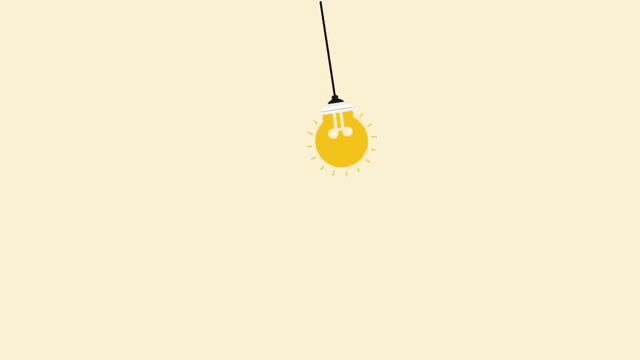 That's why understanding intrinsic value and being able to accurately assess it is so important. To quote Warren Buffett, intrinsic value is an all-important concept that offers the only logical approach to evaluating the relative attractiveness of investments and businesses. Now, truthfully, we simplified things with assumptions to illustrate the concept. 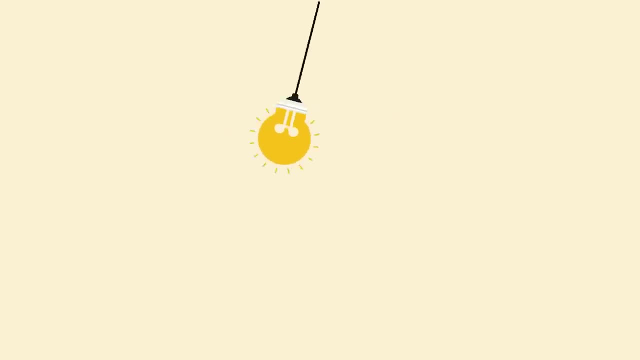 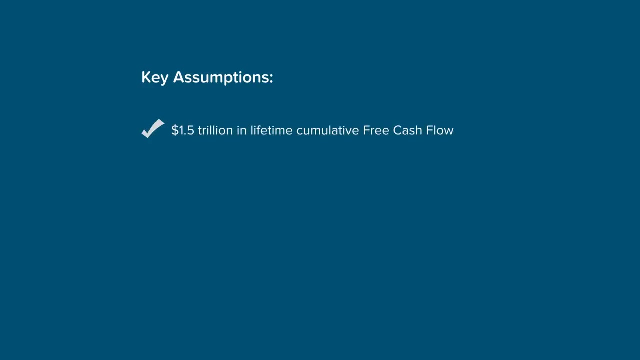 In the real world, the analysis needs to be a lot more rigorous. For instance, we just arbitrarily made up the number that Apple will generate $1.5 trillion of cash over its lifetime. What's the actual number? That'll depend on your investment analysis. 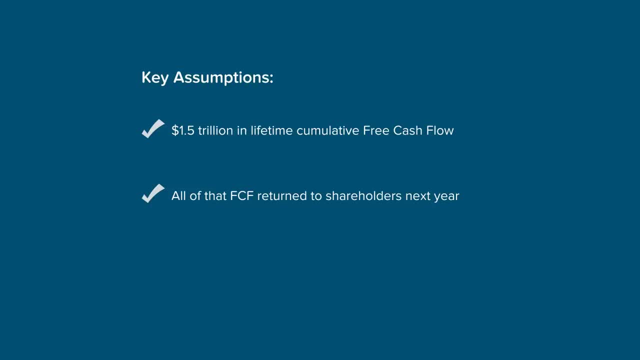 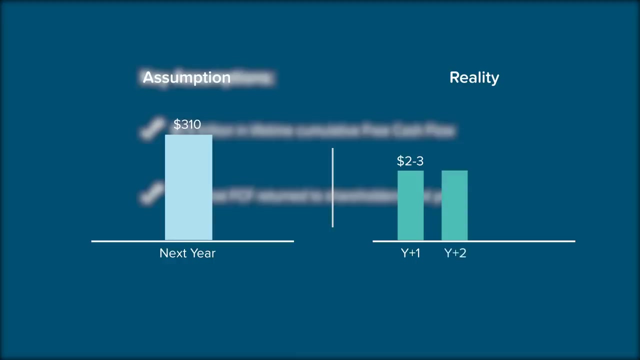 We also assumed that Apple will give you all of the $310 per share of free cash flow one year from now. Realistically, that's probably going to be spread over multiple years. For context, right now it's giving shareholders back $2 to $3 per share a year through dividends. 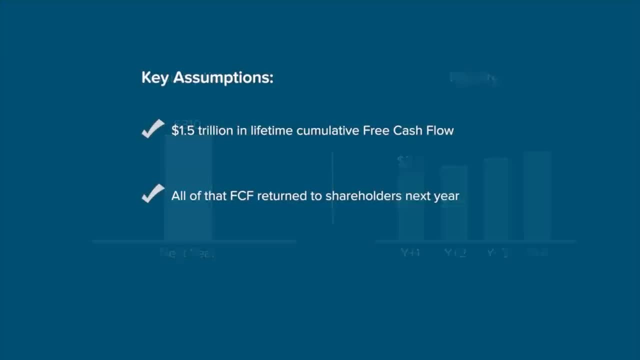 So the timing will be spread out over multiple years. How would this timing impact your valuation? We also assumed that we would target 10% return a year. Is that a good return that's commensurate with the risk we're bearing? How do you tell? 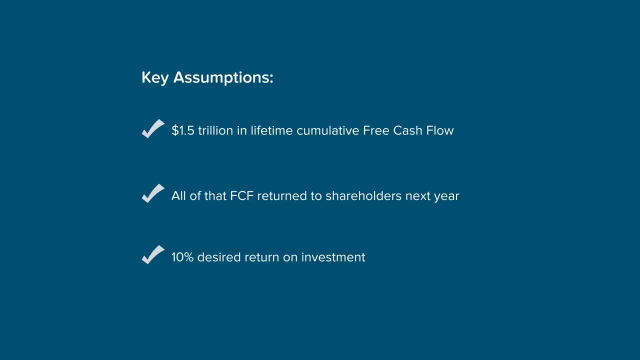 All of these will impact the true intrinsic value of the stock. We also assumed that we would target 10% return a year. How do you tell All of these will impact the true intrinsic value of the stock? We also assumed that we would target 10% return a year. 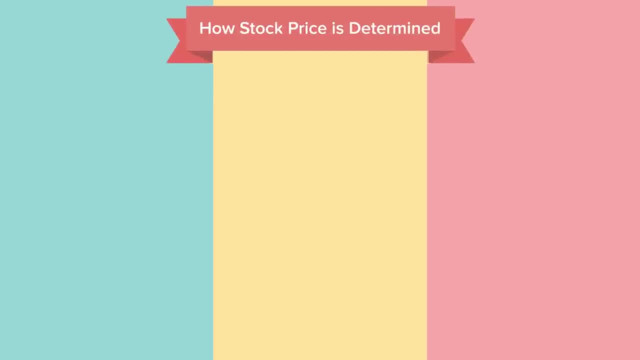 We also assumed that we would target 10% return a year. We also assumed that we would target 10% return a year. That's conceptually how the stock price is determined. Both the buyers and the sellers of a stock perform a rigorous investment analysis to